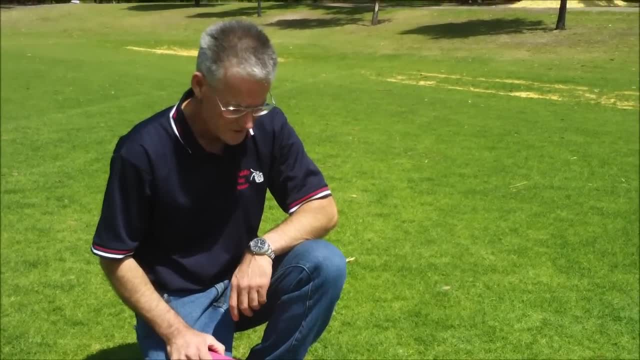 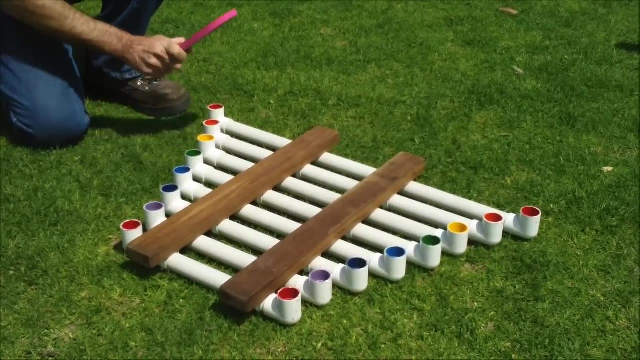 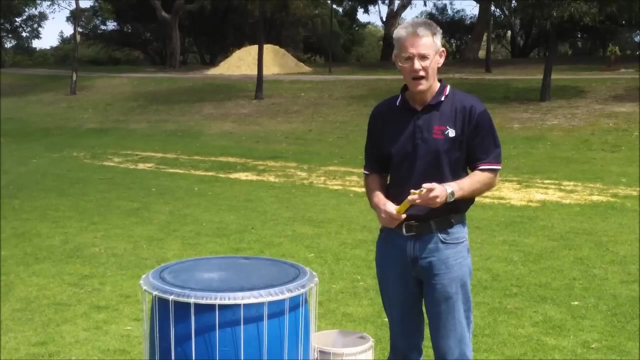 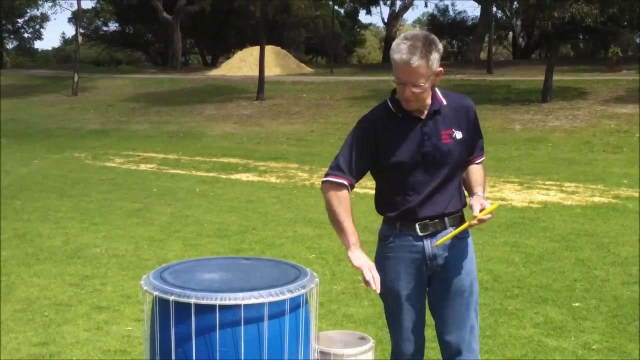 at the same time facing each other, which is lovely for kids playing together. It's much quieter than the big bass-domophone. I've got 16 different drums and these are just three of them. Most of them are made from recycled materials, like this big barrel and this big PVC container. 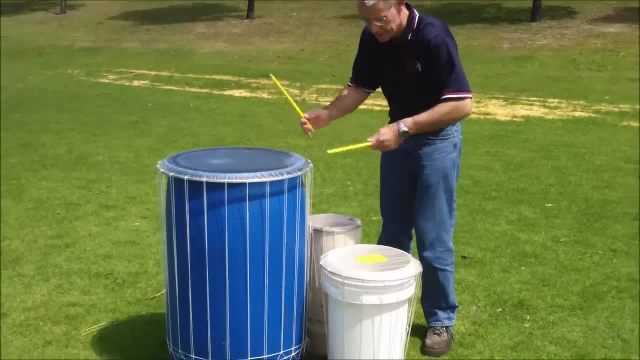 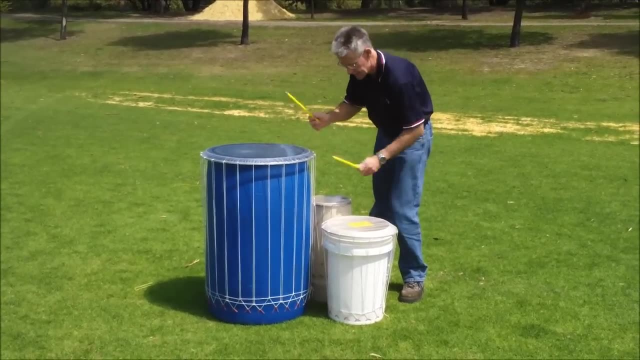 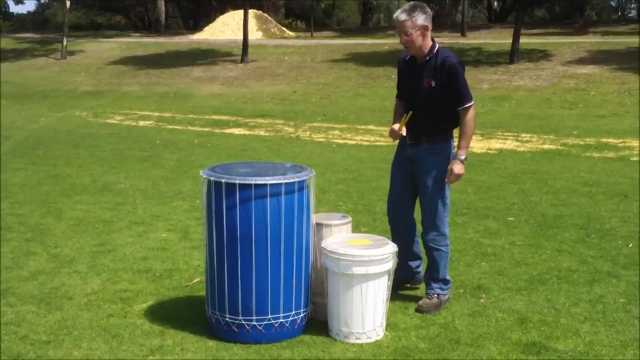 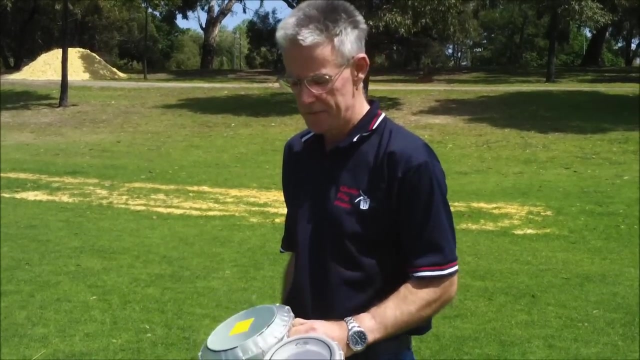 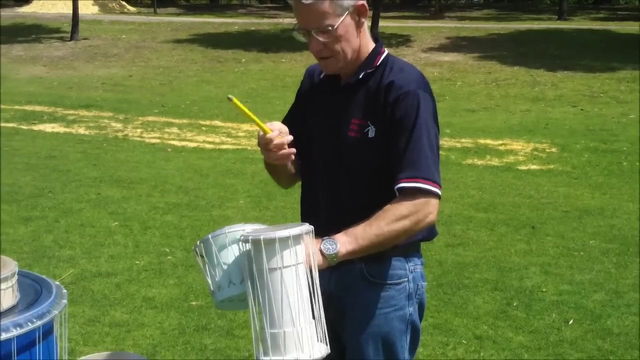 and actually they sound pretty good And I think they sound wonderful. in fact, I don't just have huge drums, of course. I've also got little things like bongos and African talking drums. Now, your African talking drum is pretty cool. 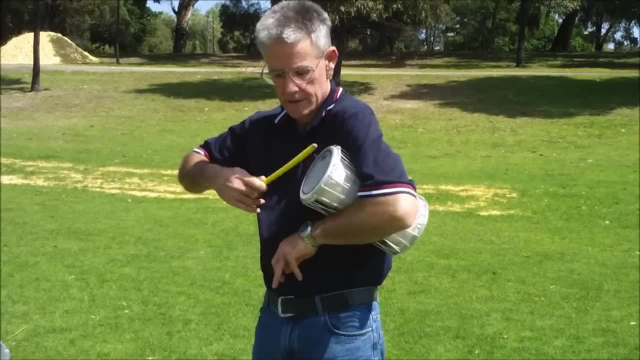 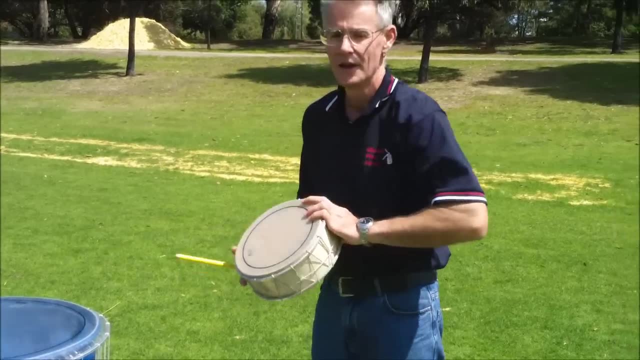 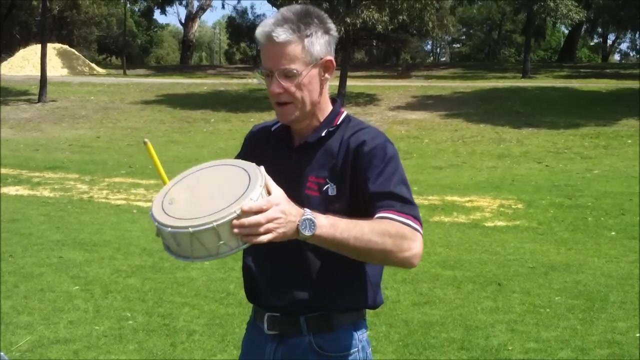 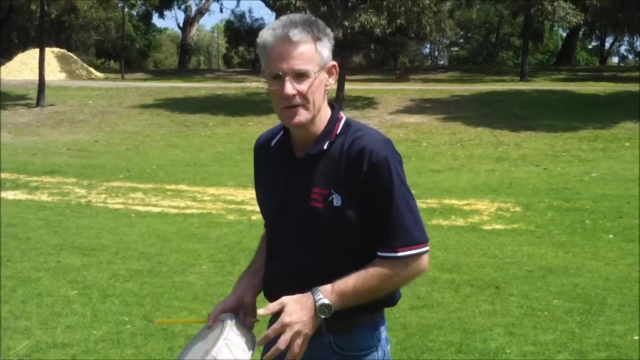 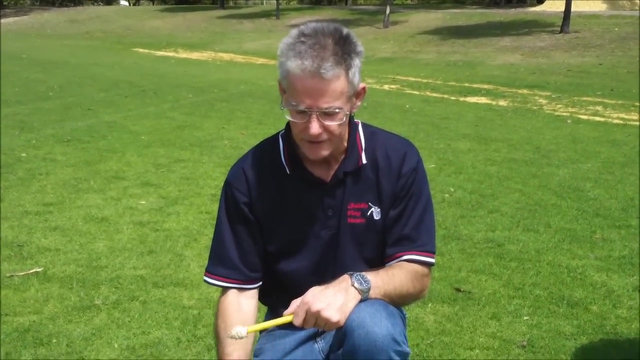 And I've also got ocean drums, which is also an amazingly loud snare drum. That's just some of my drums. This is a metallophone. It's made from recycled aluminium and PVC pipe and it's based on the Indonesian Gendair. 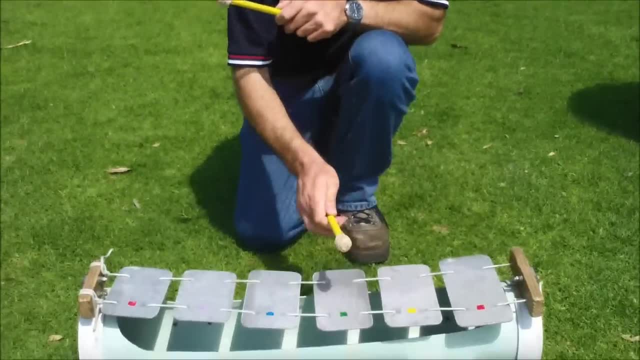 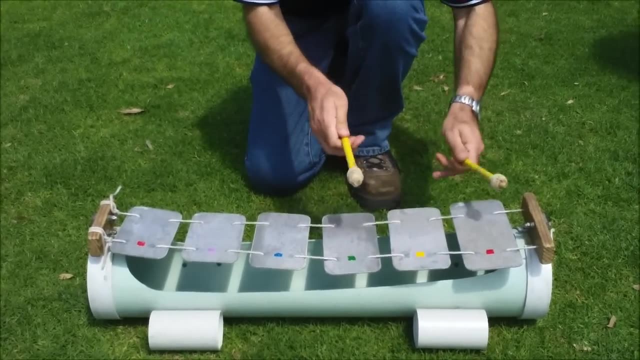 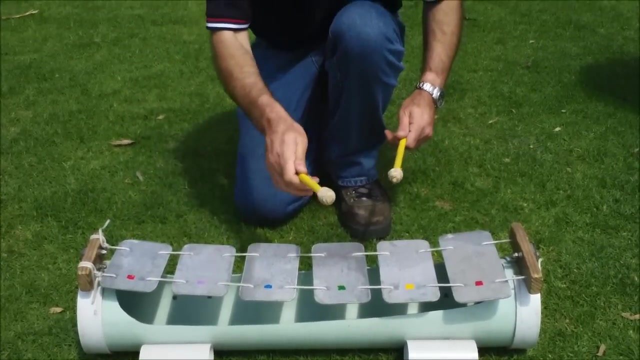 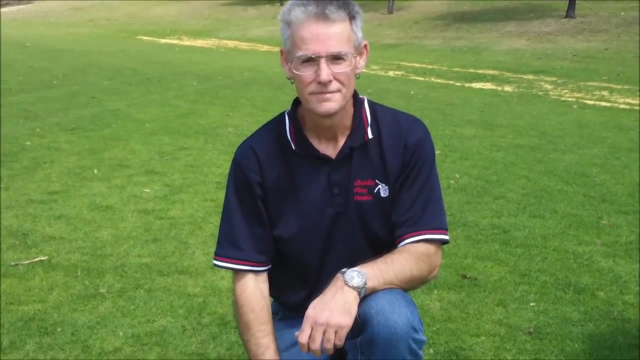 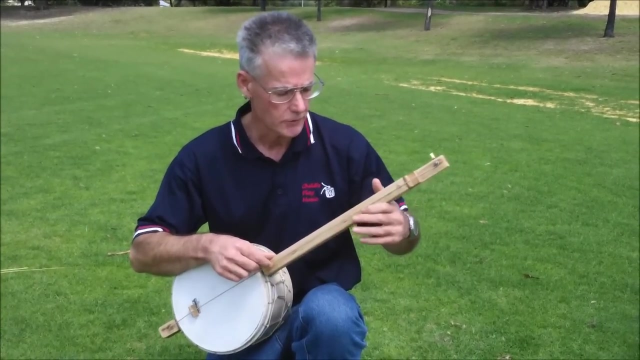 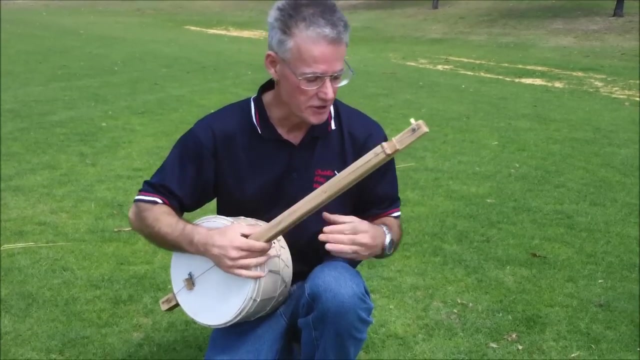 It's an interesting little instrument because it's got an unusual scale. This is one of my bass banjos: single-stringed and fretless. You can play it plucked, of course, Which is a pretty interesting way to play it, Or you can play it with a bow. 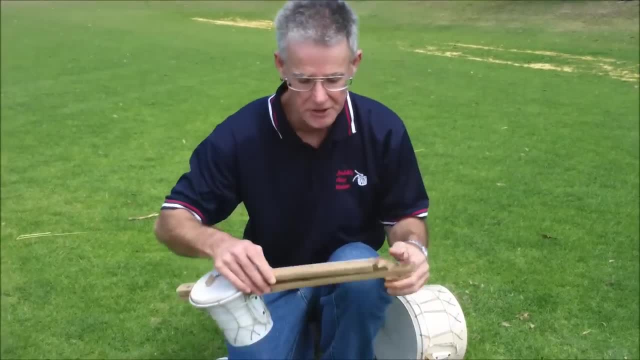 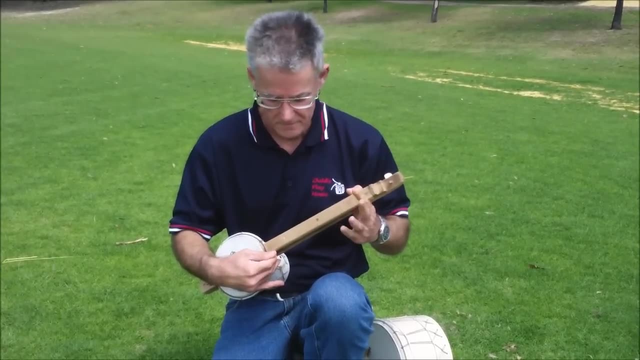 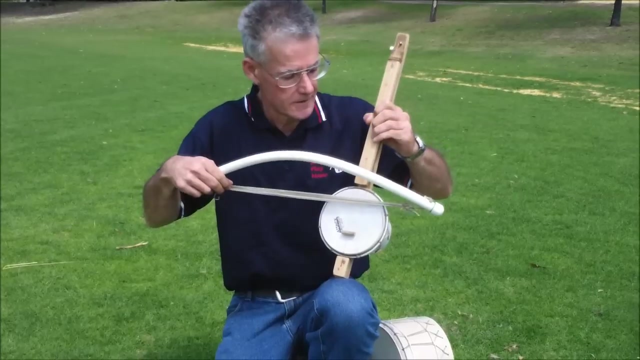 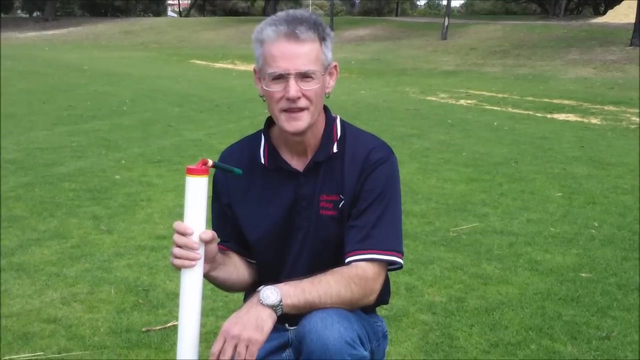 Bass banjos are fairly unusual. A treble banjo is a little bit more usual And, yep, you can play that with a bow too. I've also got wind instruments. This is a lovely little thing called a balloon bassoon. 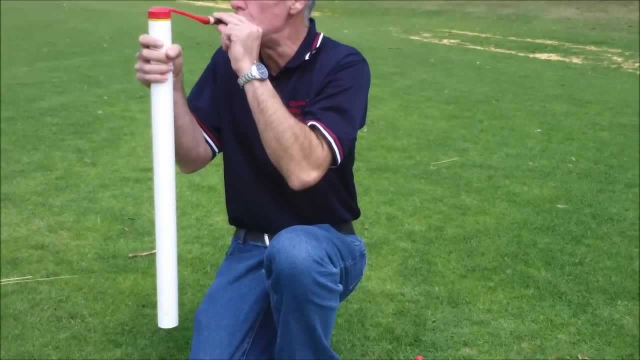 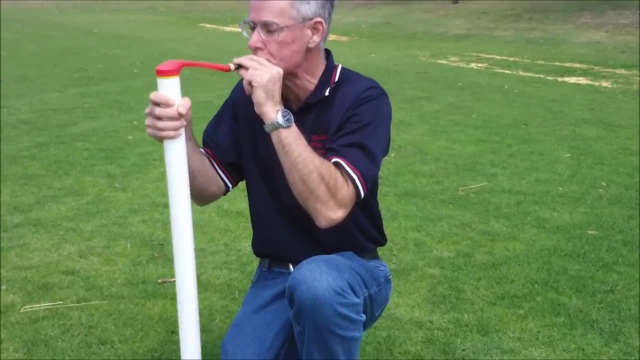 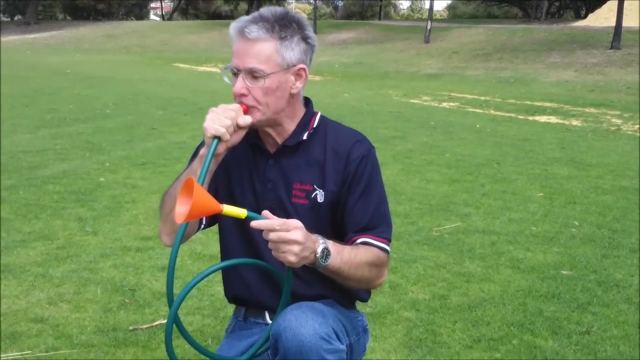 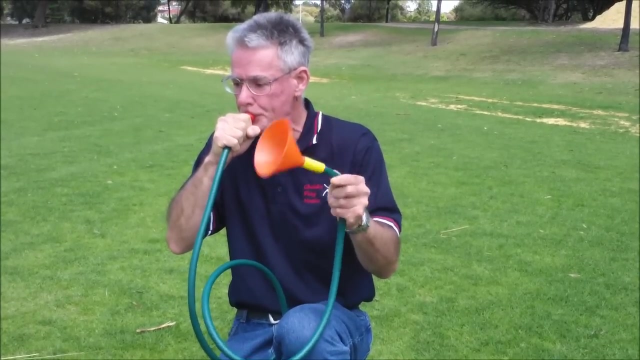 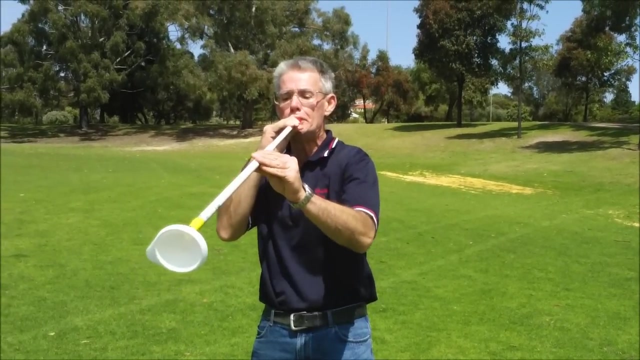 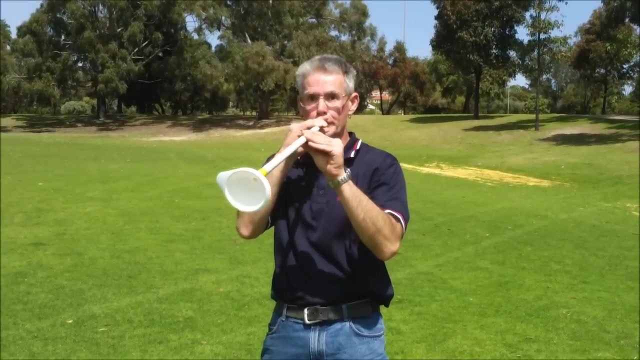 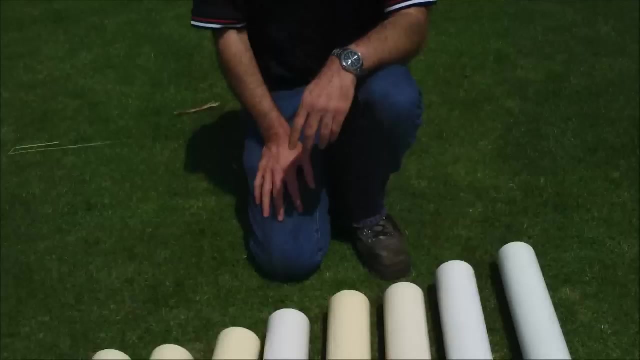 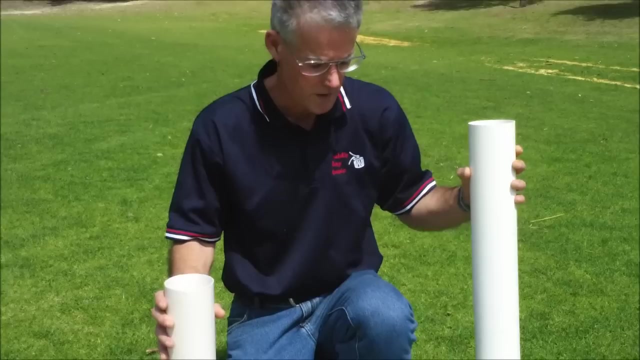 It only plays one note. That's pretty cool. Garden hose trumpets. This is a slide trumpet, rather like a trombone. It's a little bit more …. I'm no trombonist. These are stamping tubes. They're based on instruments from Papua New Guinea. 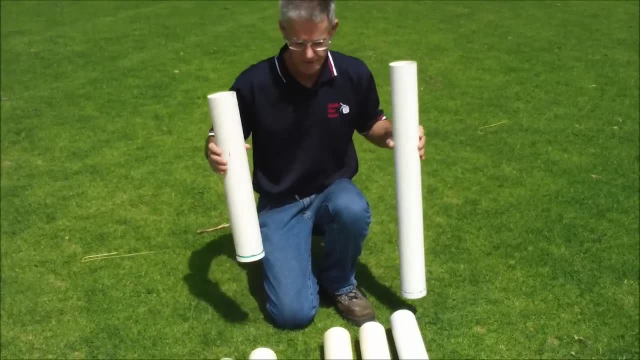 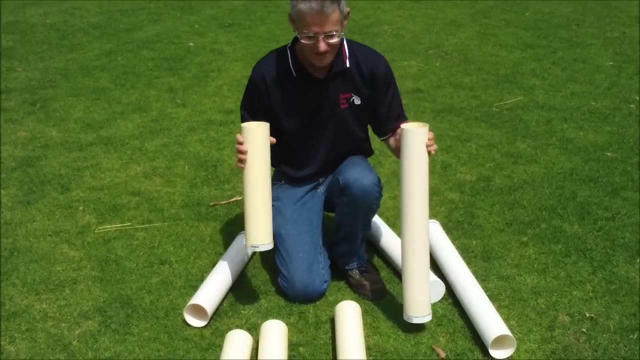 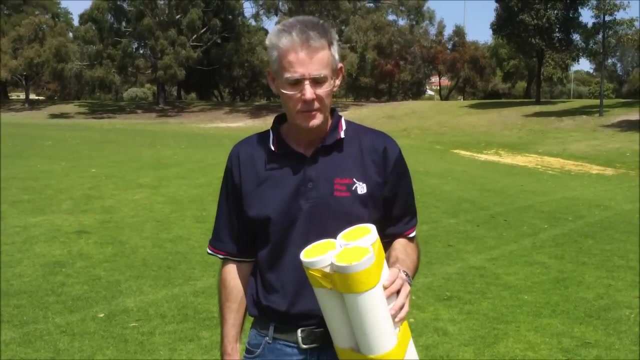 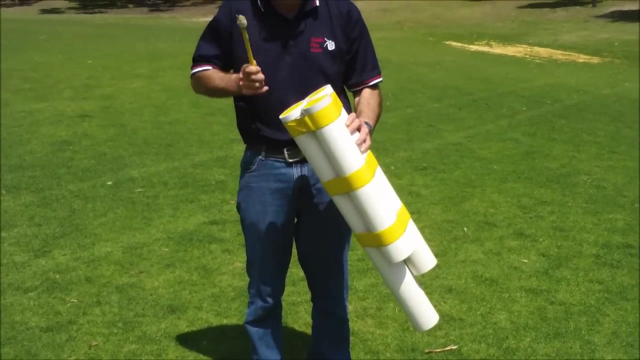 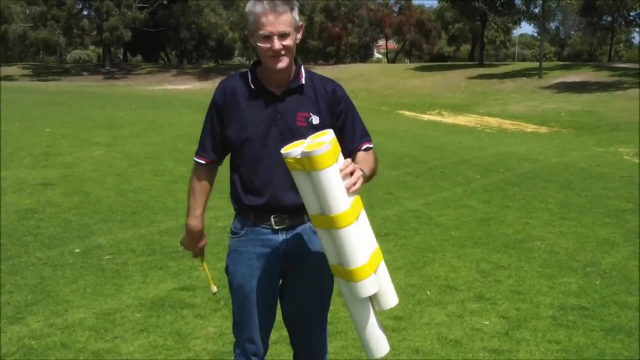 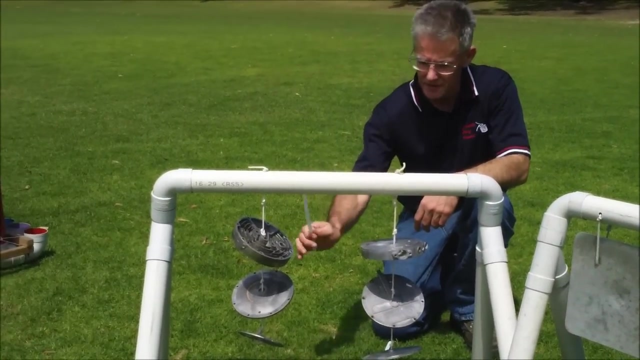 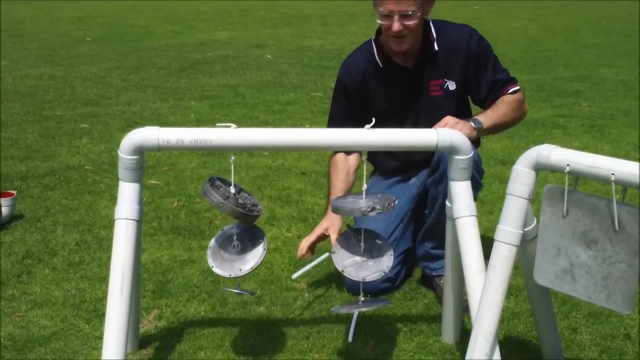 where they make them out of big bamboo. This one's made from three stamping tubes, but you can play it with a drumstick. it's called boobams. This is a bell tree made from recycled aluminium castings, and these are gongs made from recycled aluminium.